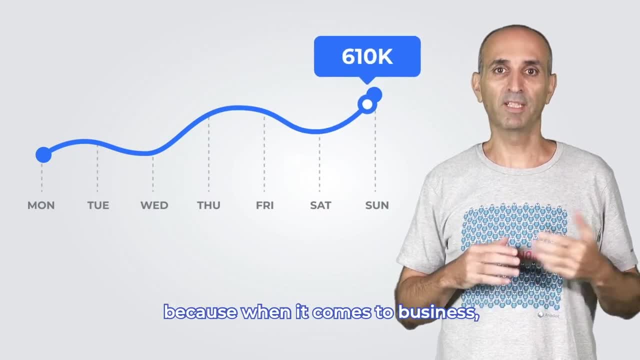 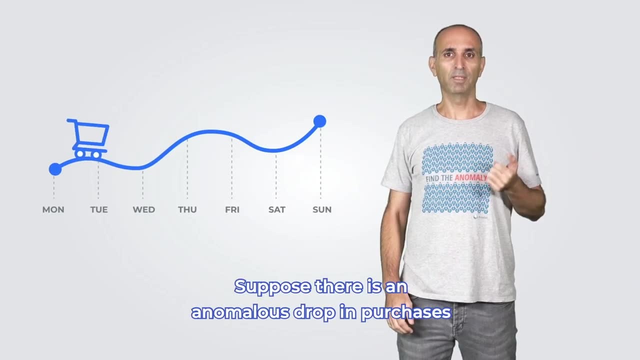 in time series. data is especially valuable to business because, when it comes to business, anomalies often point to areas that need attention. Let's take an online store. Suppose there is an anomalous drop in purchases of a particular product. Maybe they ran out of stock? 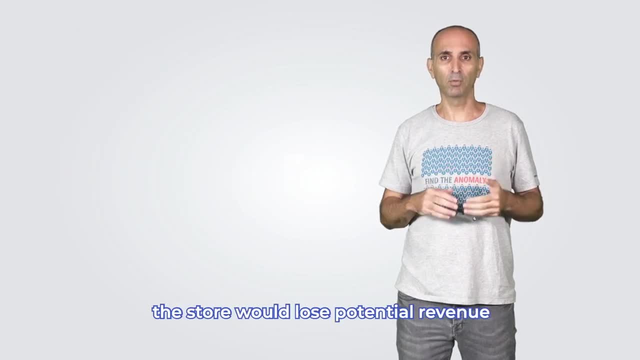 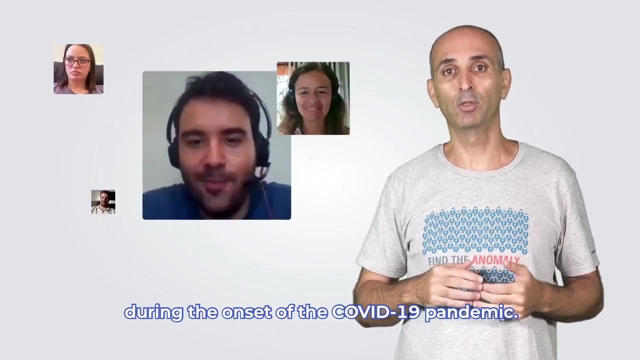 If this anomaly went undetected, the store would lose potential revenue and customers who may not return. A great example of a business anomaly happened during the onset of the COVID-19 pandemic, As droves of people began working from home and started videoconferencing they created. 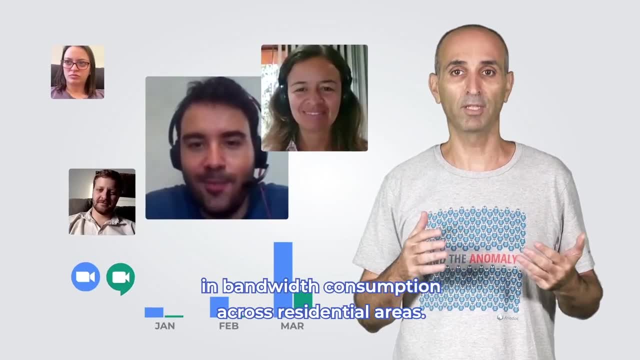 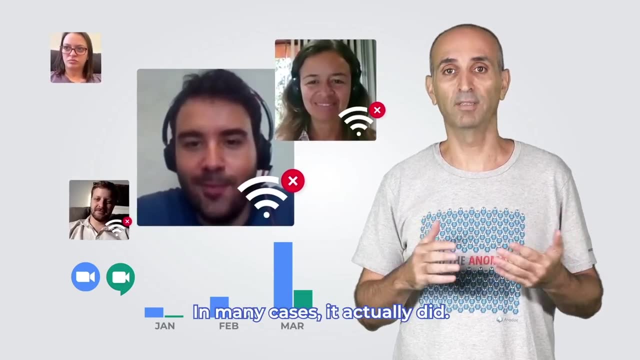 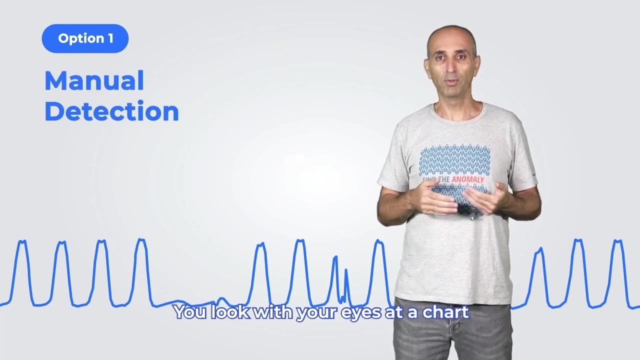 an anomalous spike in bandwidth consumption across residential areas. If telcos did not respond, their quality of service would have suffered. In many cases it actually did. So how do you detect for time series data? Well, the simplest way is manual. You look with your eyes at a chart of a. 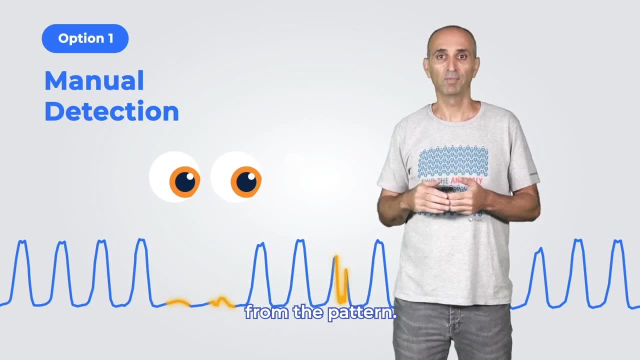 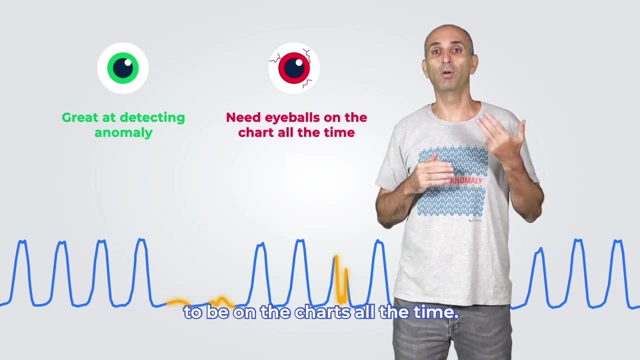 time series and you find where the data deviates from the pattern. Our brains are great at detecting anomalies, but you need the eyeballs of a person to be on the charts all the time. A more automatic way is to use an alerting system based on simple statistical rules or static thresholds that have 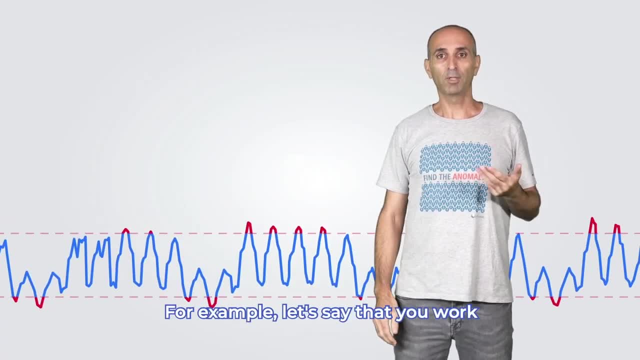 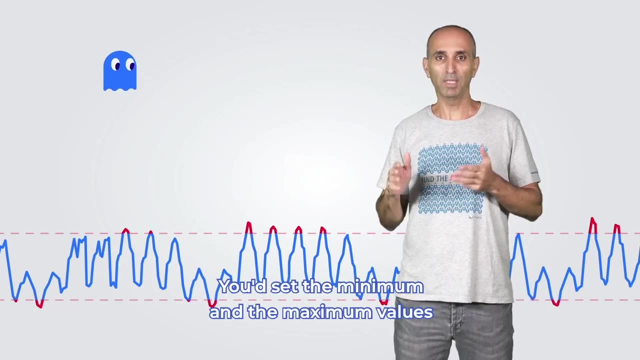 to be manually adjusted. For example, let's say that you work for a gaming company and you know that revenue from in-app purchases is not going to be the same as the revenue from the purchase of a game. You'd set the minimum and the maximum values and only get alerted when revenue exceeds. 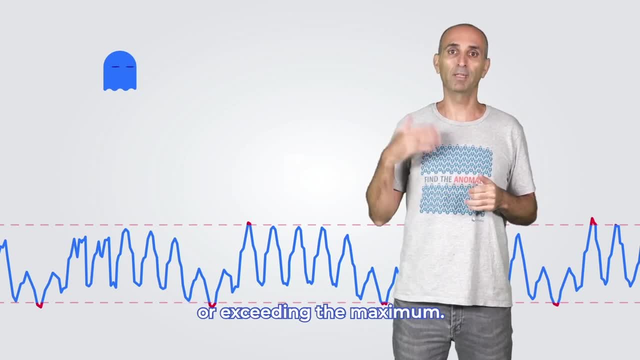 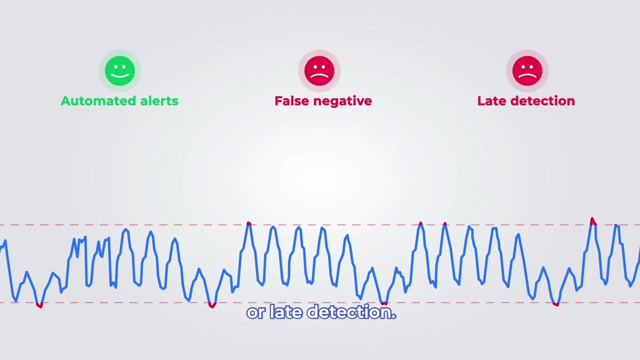 those limits, either by dropping below the minimum or exceeding the maximum. Here you've got the advantage that your alerting is automated, but the disadvantage of false negatives or late detection. You would also get false positives when the KPI's pattern changes, For example if a game becomes 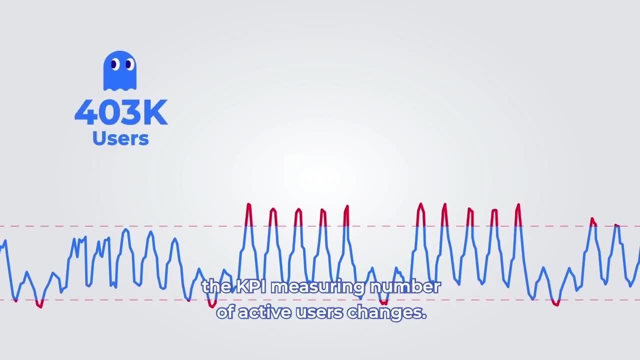 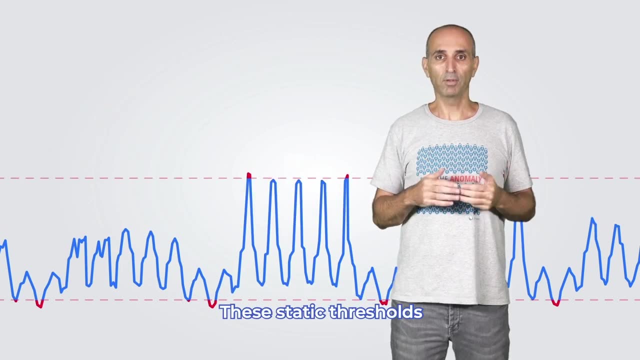 popular. the KPI measuring number of active users changes and a static threshold alert would send a lot of false positives unless it is manually fixed. These static thresholds can be slightly improved with simple statistical rules such as alert me if revenue drops by 20% compared to last. 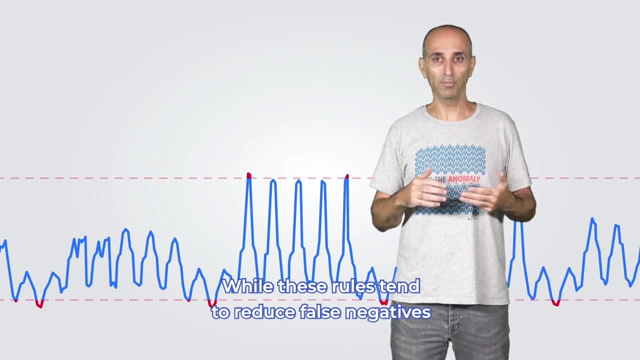 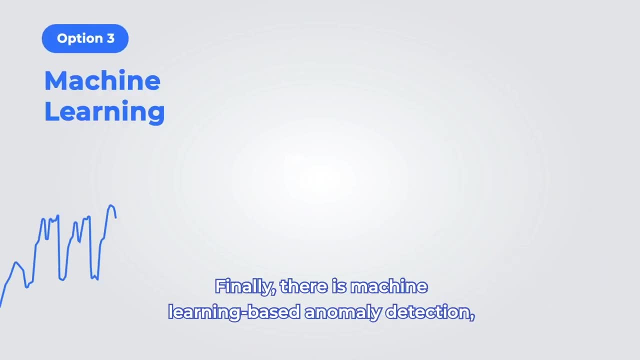 week's average. While these rules tend to reduce false negatives, compared to static thresholds, they often generate a lot more false positives. Finally, there is machine learning based anomaly detection, which is a system that uses machine learning algorithms to learn the normal patterns in the data, accurately detecting all the false negatives and the negative ones. You can also